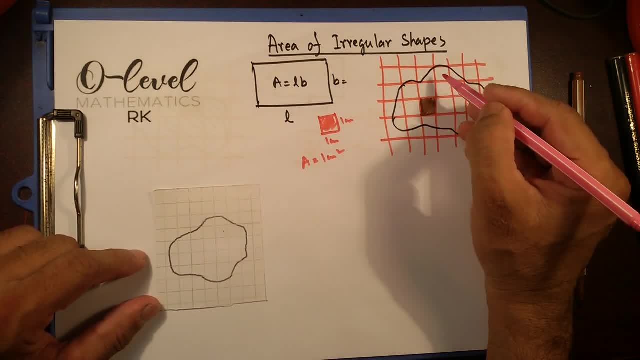 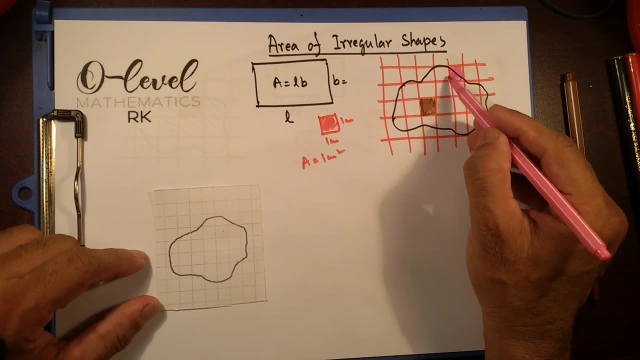 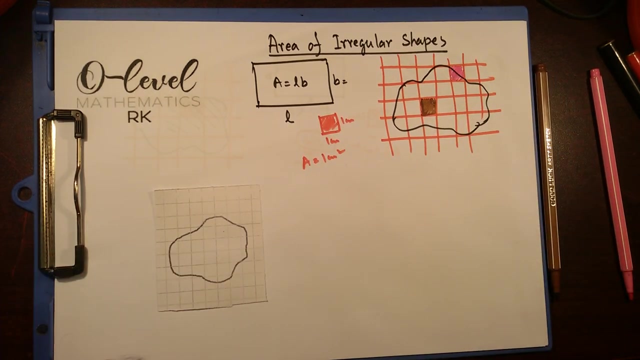 Square that goes on the, on the shape. We're going to color it in pink. Okay, See that It's. it didn't cover the whole square, It's cover the sum of the part, Okay, Some of the part. whichever square cover, We're going to pink it by a color pink and rest of them that complete one. We're going to color it with blue and brown. 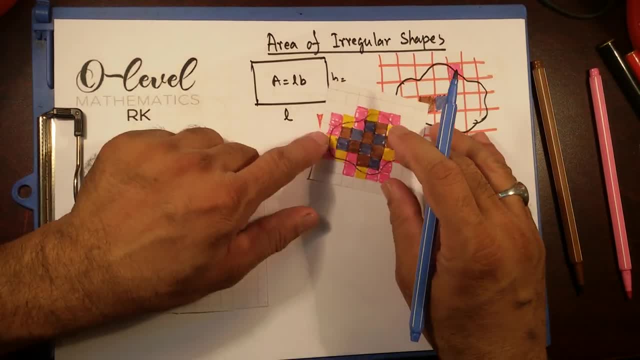 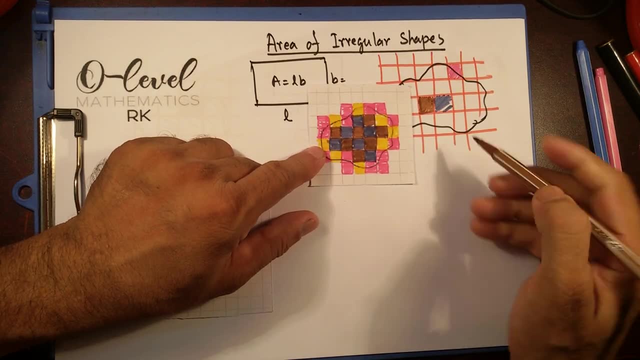 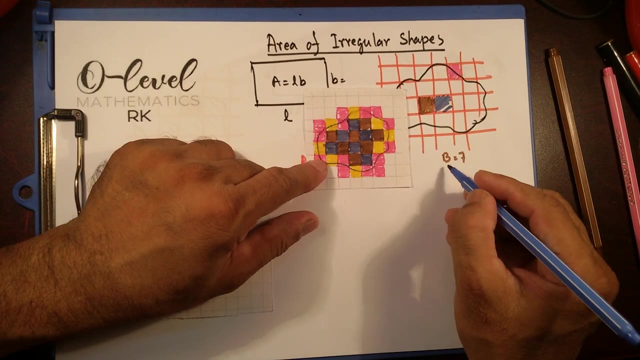 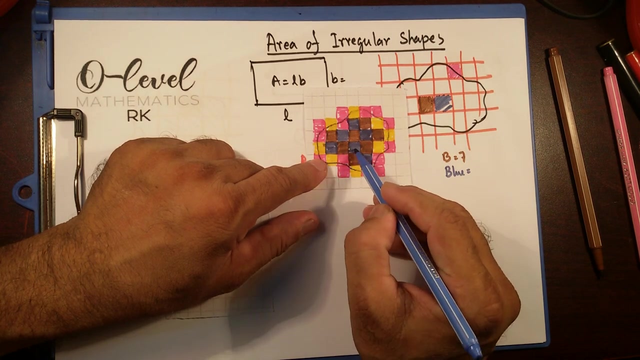 Okay, I have done this one for you. Okay, Look at this. All the brown, There are one, two, three, four, five, six, seven brown, brown, brown squares, That's completely fill this space is seven. And then, okay, Brown blue. So I'm going to write down: blue blue: one, two, three, four, five. one, two, three, four, five, six, six. So total seven plus six is seven. 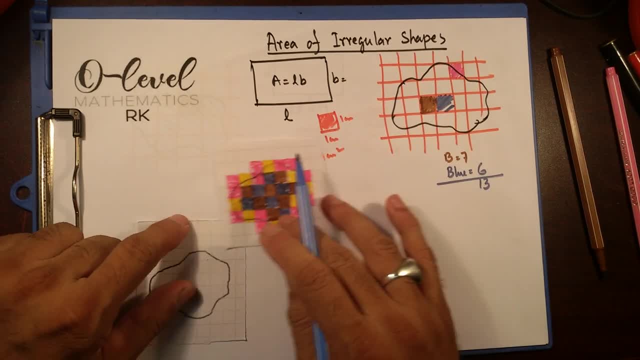 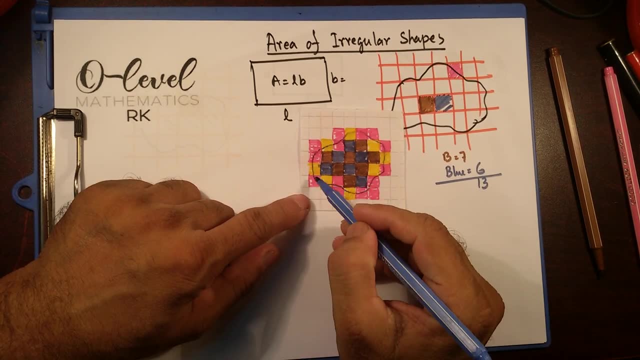 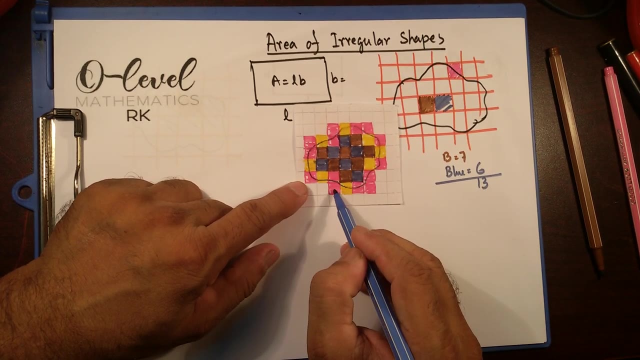 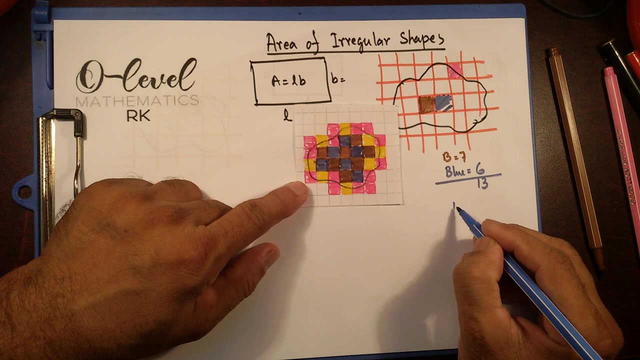 Thirteen complete square. What about those pinks? one, Okay, Let's. let's count all the pink one: This pink square is not filled. the the whole square inside there is partially filled, So I'm going to count them. One, two, three, four, five, six, seven, eight, nine, ten, eleven, twelve, thirteen, fourteen. So fourteen pink, one, pink fourteen, And alongside 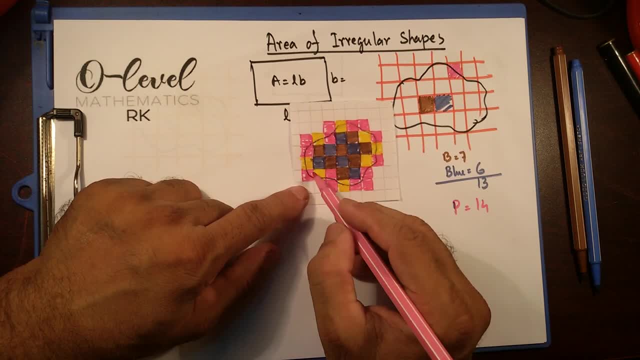 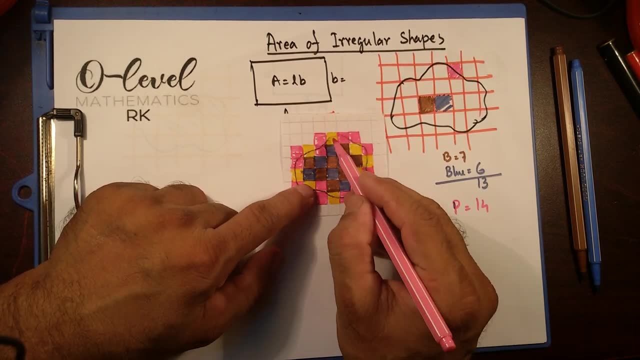 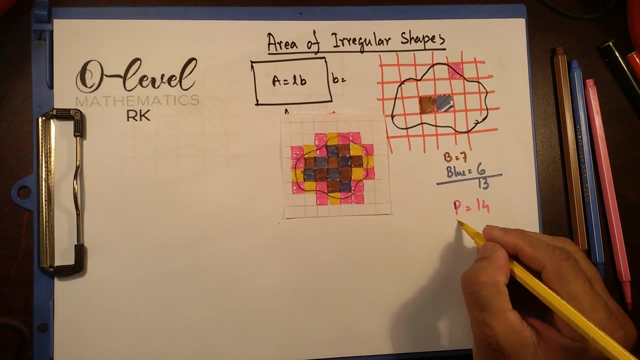 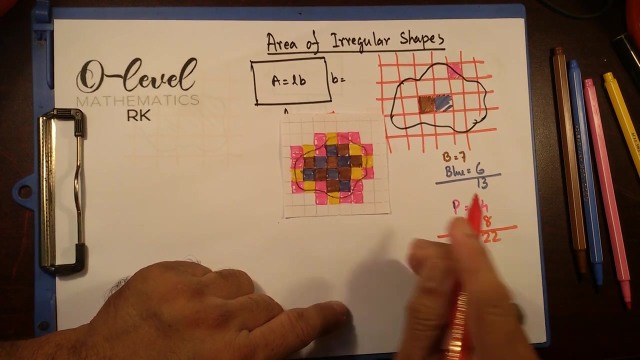 of this. I use actually yellow color as well to color those that go through all the way. So yellow one. one, two, three, four, five, six, seven, eight. So it's eight yellow yellow- I got a yellow one over here, So yellow is- I don't think you can see that- yellow- equal to eight of them. So fourteen and eight is twenty two. So this area, Okay, The very interesting way Calculate. 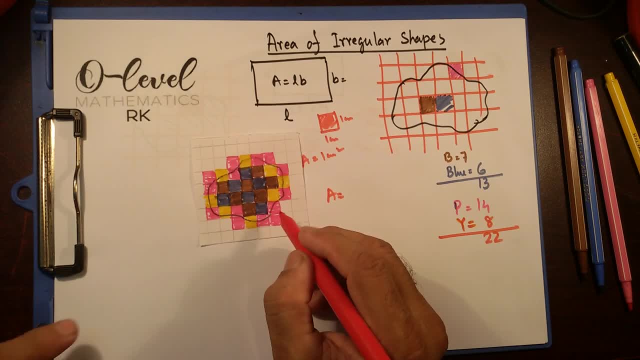 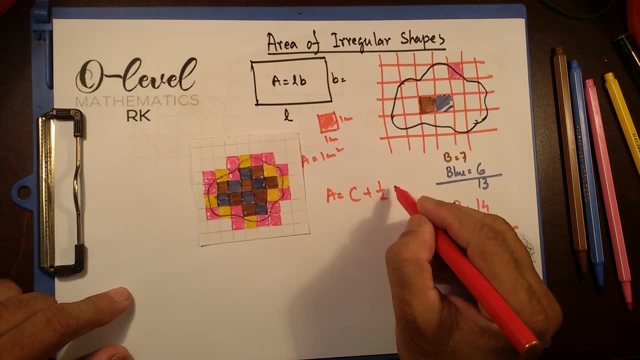 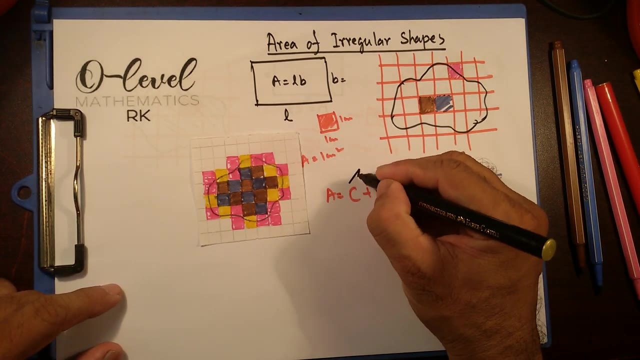 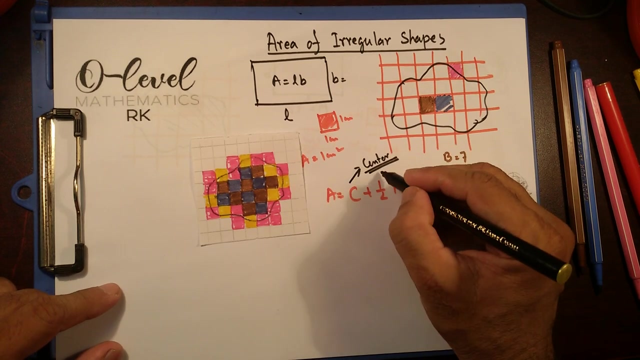 calculate this area, Everything. Okay, Let me write down the formula the way it goes: first C plus half, then P, What that actually means. This C means? this C means that goes through the center of this area. center or inside, Okay, Inside the area, Let's put that inside- completely filled inside And this and this: 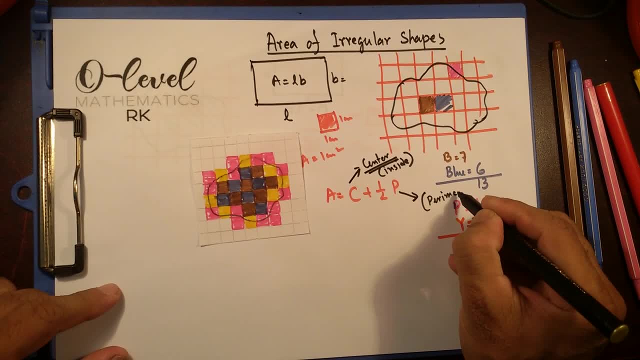 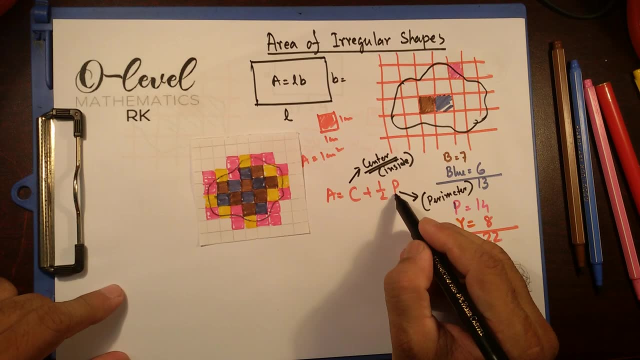 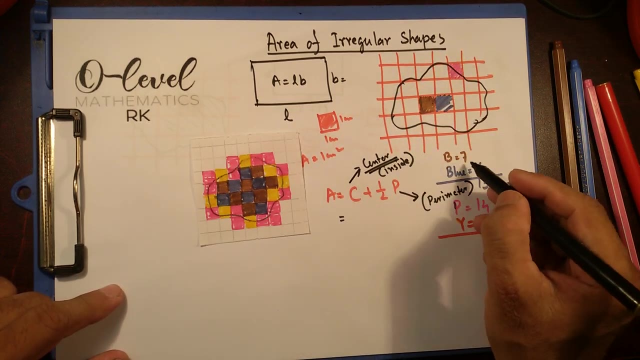 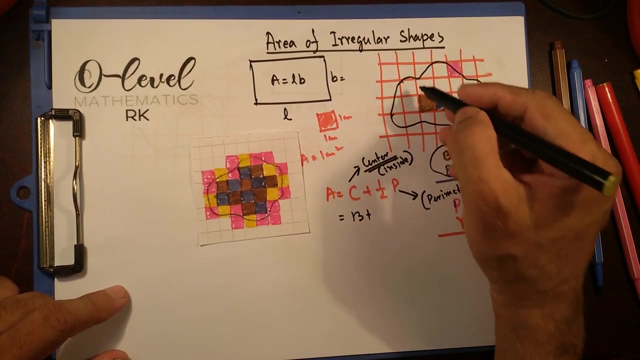 P is on the perimeter. Okay, Perimeter So squares, number of squares that are inside the shape and number of squares that on the perimeter, So number on the inside, the center or inside, there is total thirteen And we are taking average of this outside on on the perimeter, That's twenty two half times twenty two. So if I cross this one, 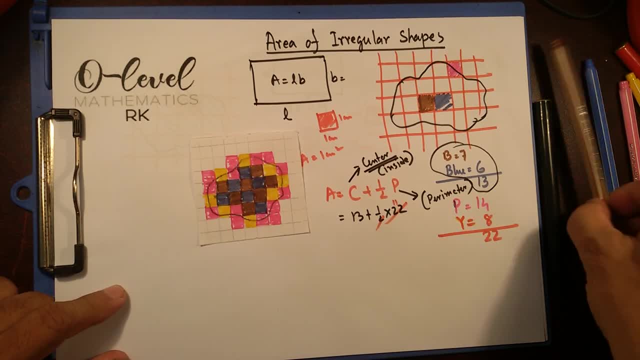 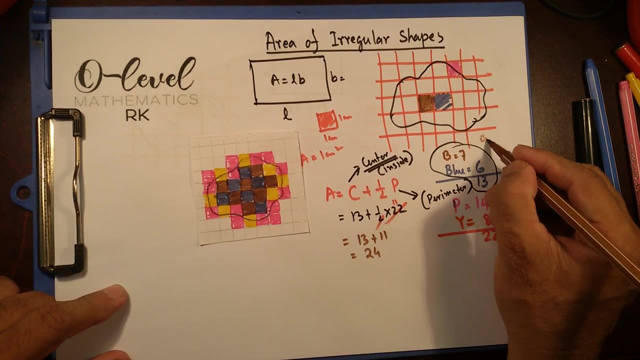 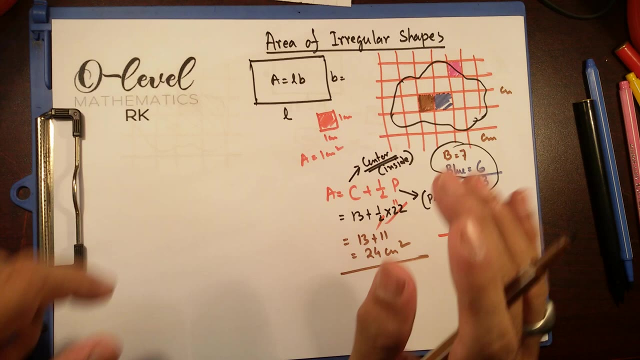 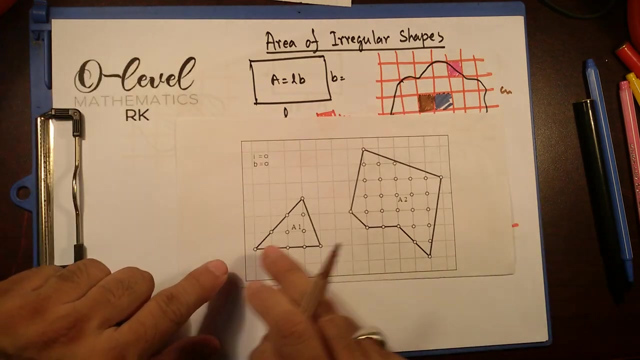 Out is going to be eleven, So I end up with thirteen plus eleven, equal to twenty four. If this is centimeter, Yes, I told you before centimeter, centimeter, So it's square centimeter, That's irregular shapes area. Okay, This is one way to do that. Another way is a fixed theorem, That's another mathematician. I have this: two spaces, Okay, Let's say I and B. Okay, I is in the. 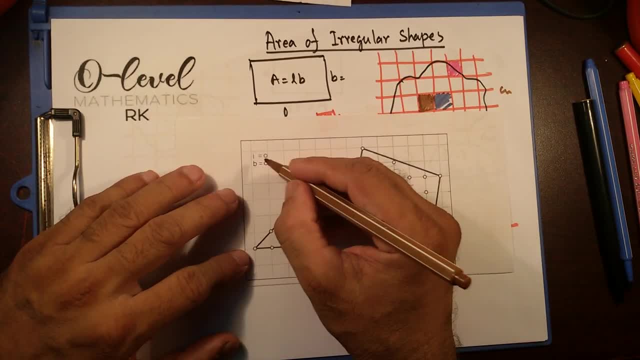 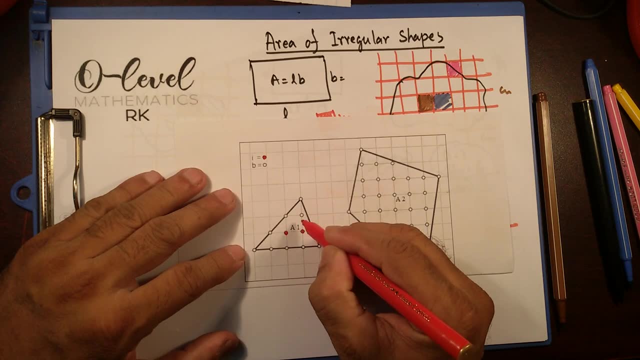 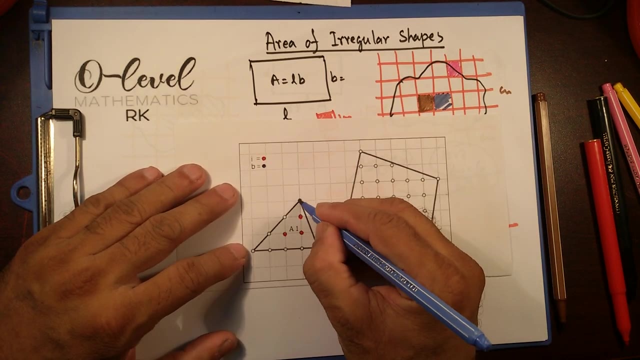 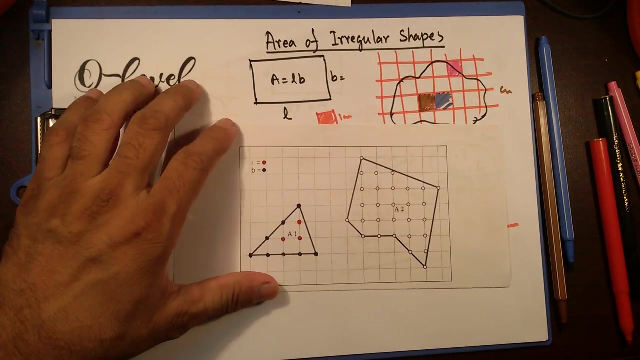 inside the space, inside the shape. Okay, Let's color that inside that color with red. So these are red, Okay, And everything that's on the boundary by blue. One, two, three, four. It does look like probably black, but it's actually blue, Okay. The peaks formula. Let me write down this peaks formula. Okay, It's called. 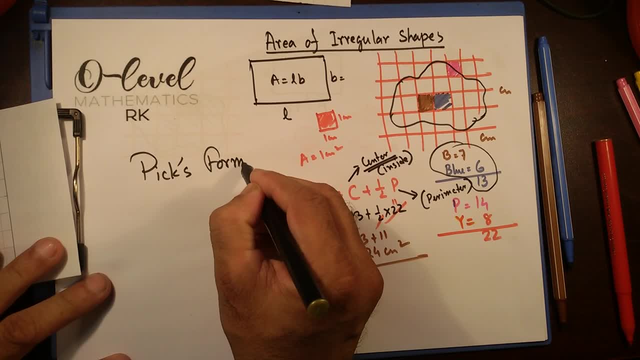 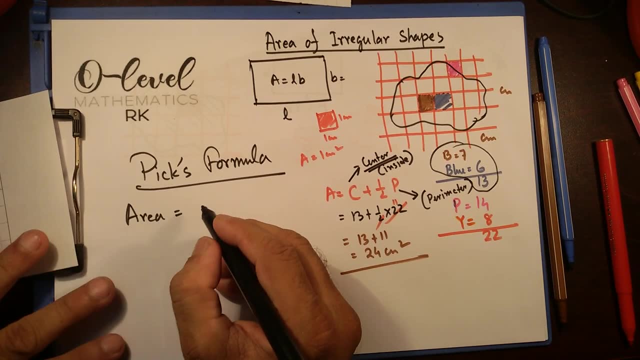 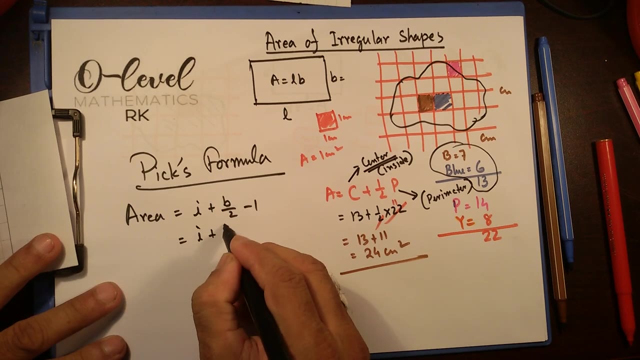 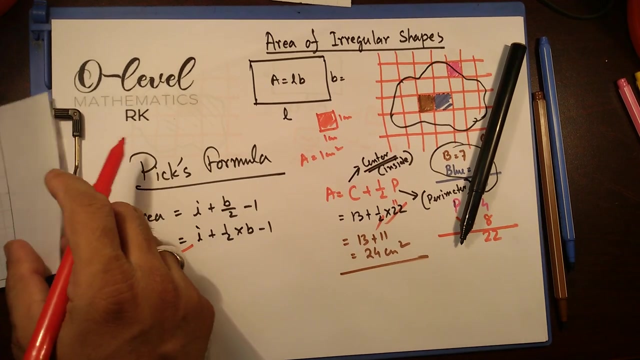 peaks theorem or peaks formula. I'm going to write down formula for the time being And it goes: area required: area Area equal to the formula. goes I plus B by two minus one. Or you can say I plus half times B minus one. This I, I is the inner point. Okay, How many points inside the shape? Okay, Particularly this one I have. 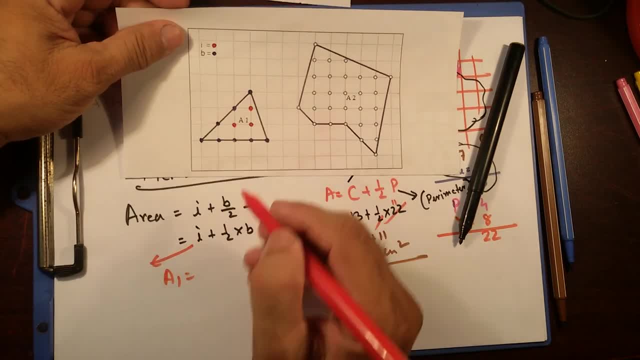 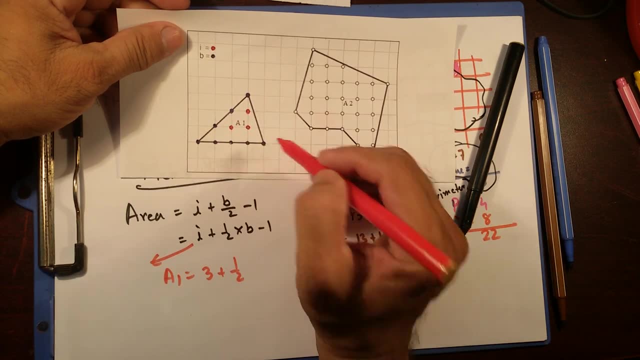 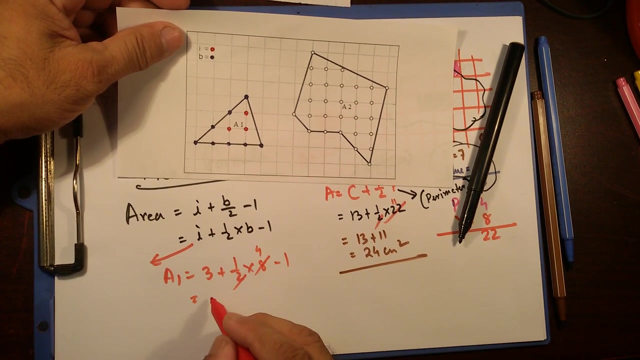 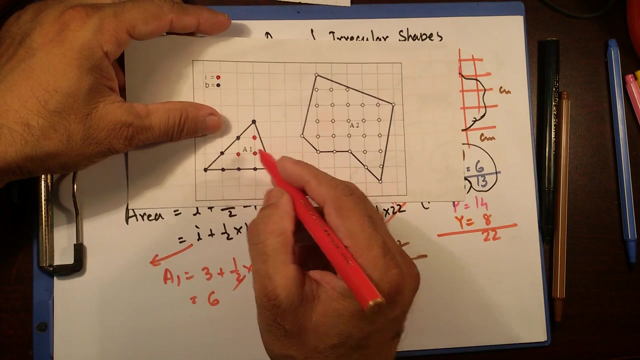 Okay, Area one. I have inner point three And then half B on the boundary. one, two, three, four, five, six, seven, eight. It's eight minus one. So that cross it out four. So three plus four, seven, seven minus one is six. Now I think you know the area of the triangle. Okay, In the next video I'm going to show you how to calculate, how to find out the area of triangle. But right now, 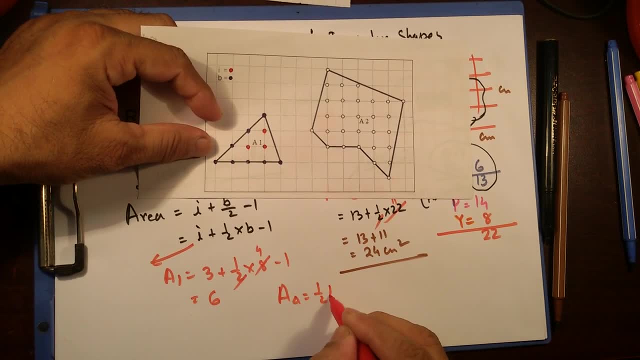 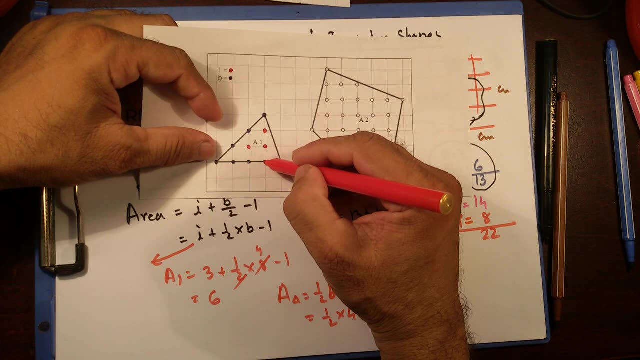 Now, whatever you know, area of triangle equal to half base into height, So half base over here, 1, 2, 3, 4, that's 4 units And height 1,, 2,, 3, 3.. 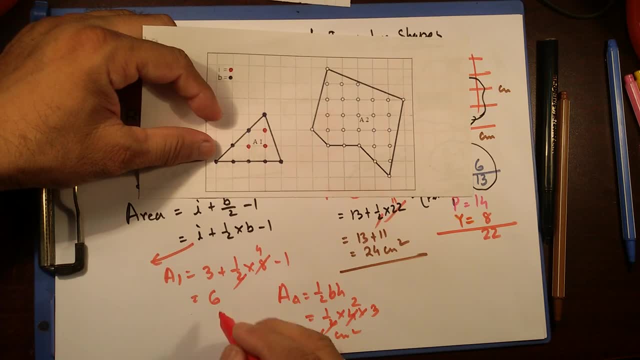 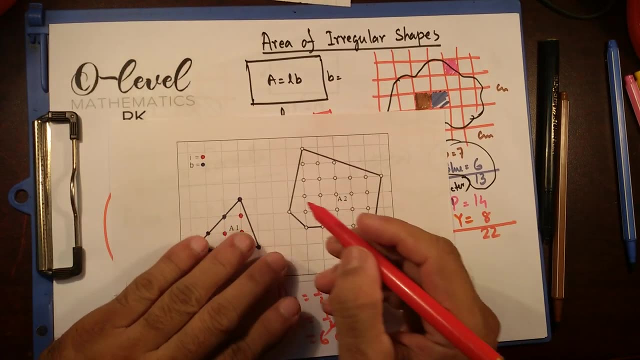 So that's going to be equal to 6 square centimeter, And that was 6 square centimeter by using the Peck's theorem. okay, So let's see if it works for this one or not. Red one inner point. I'm going to mark it with red, okay. 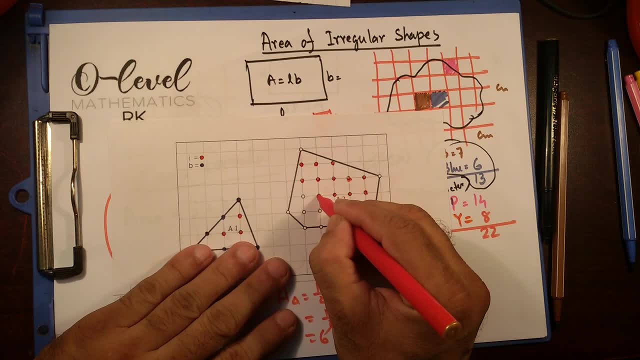 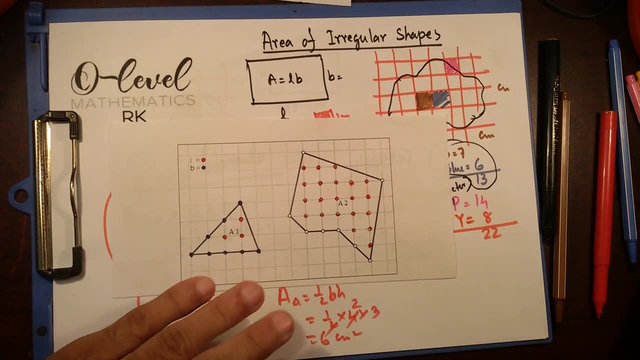 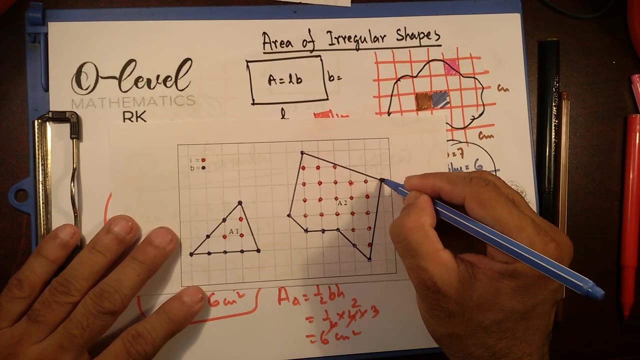 This is red, and then, okay, this red, red, red, red red, and probably this one too, And then with blue: 1,, 2,, 3,, 4,, 5,, 6,, 7,, 8, okay. 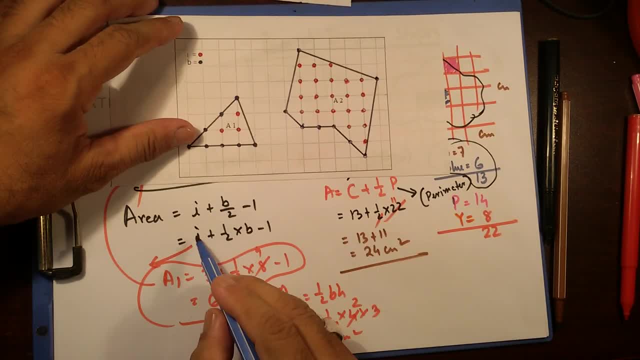 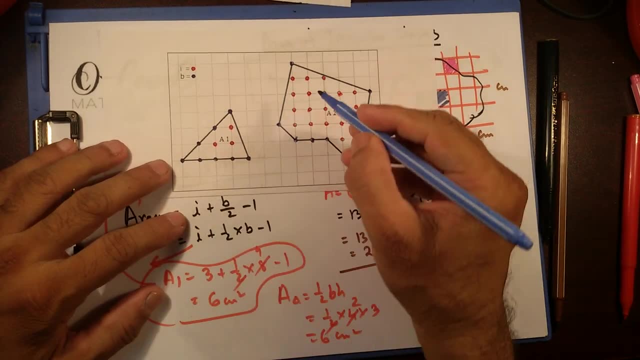 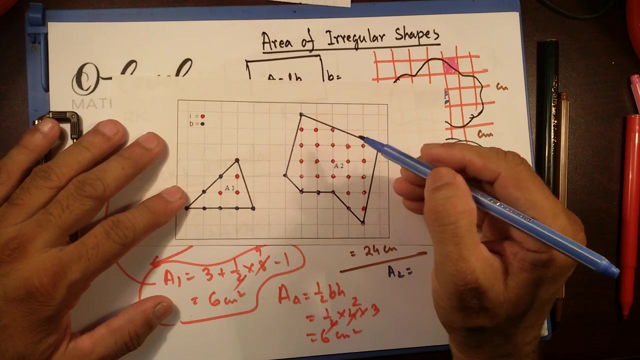 Alright, so inner, let's count that inner area 2, that one area 1.. Now area 2.. Using the formula inner points, I have 1,, 2,, 3,, 4,, 5,, 6,, 7,, 8,, 9, 10,, 11,, 12,, 13,, 14,, 15,, 16,, 17,, 18,, 19,, 20, 21.. 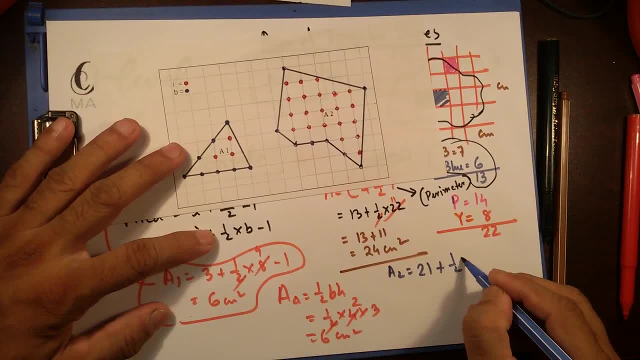 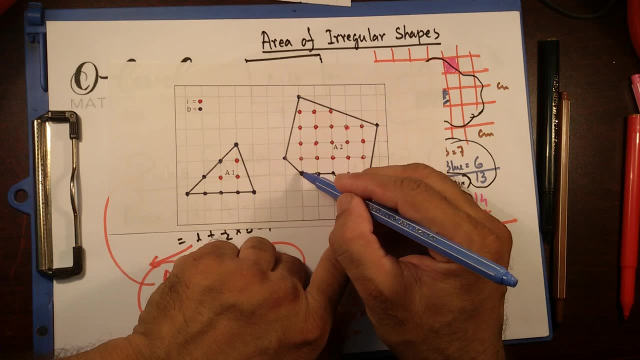 So this is 21 plus half times. B is the point of the boundary. okay, 1,, 2,, 3, I'm starting from here: 1, 2, 3, 4, 5, 6,, 7, 8.. 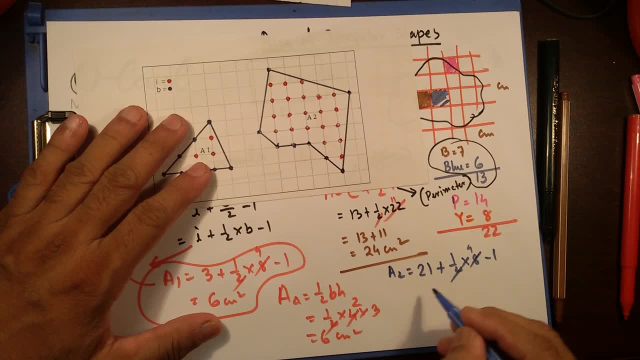 So 8 minus 1.. So that's going to be 4.. So 21 plus 4 minus 1, 21 minus 1 is 20, 20 plus 4 is 24 square centimeter. okay. 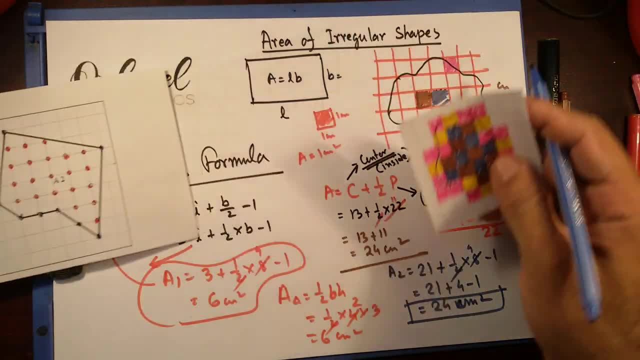 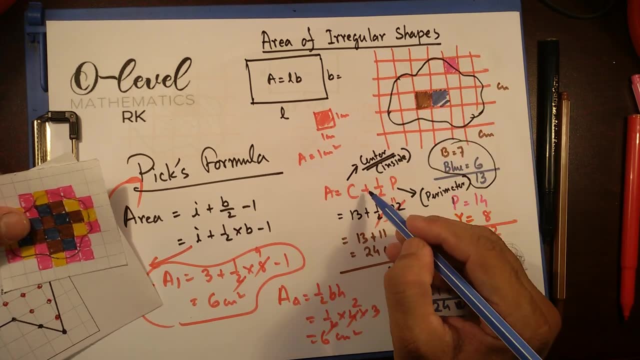 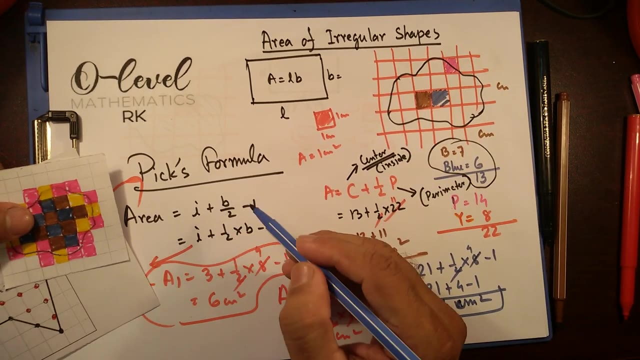 This is how we calculate irregular shape. okay, 1 is, with this formula, central complete box plus half of the box, number of box that are on the perimeter And this one inner point Plus half of the boundary point minus 1, that's fixed formula, okay. 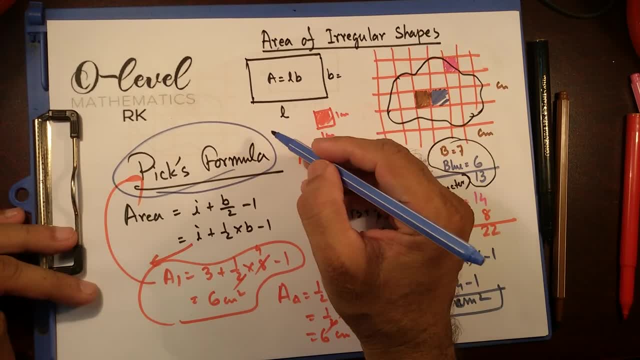 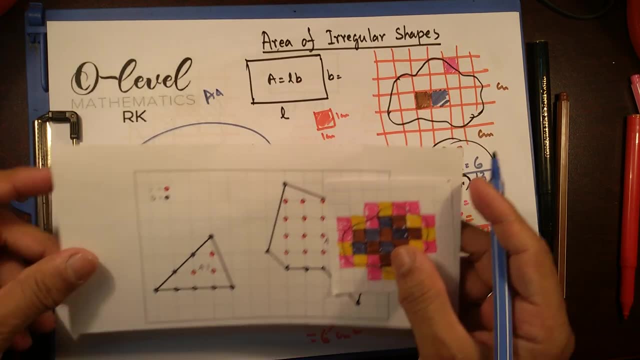 And this is how we calculate the irregular shapes. On next video I'll show you how to we how do we get area of triangle and other areas? okay, Hopefully you like it. If you do, please leave in the. leave your comment in the comment box, okay.